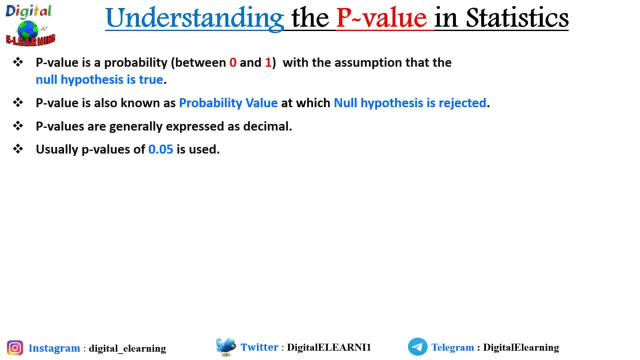 into percentage, it comes to five percent, which means that there is a five percent chance that your result could be random, that is, it would have happened by chance. on the other hand, the larger p value, say for example 0.9, means that your result have 90 percent probability of being completely. 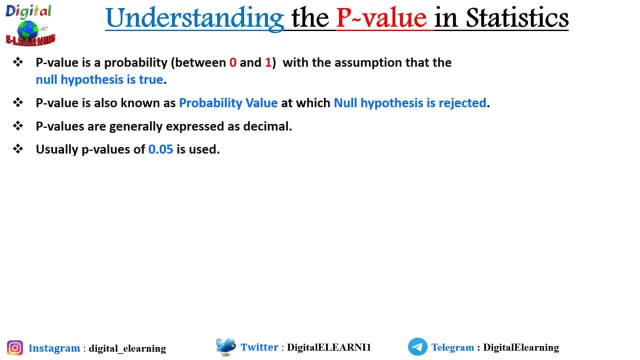 random and not due to anything in your experiment. therefore, smaller p value, more the significance your result would be. let's say, an experiment is performed to determine if the coin flip is failed or not. so if you convert this into percentage, smaller the p value is used. so if you convert, 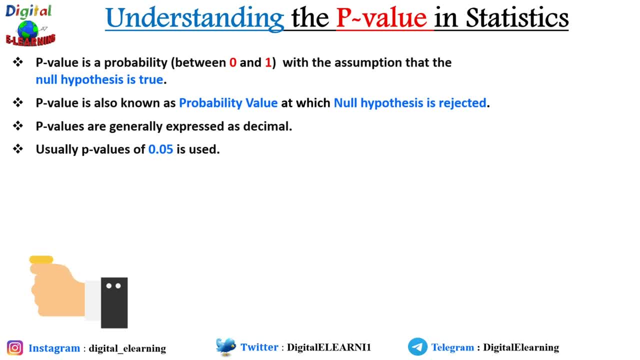 the p value 0.5. so you flip the coin, you have equal probability of getting a head or tail. that is 50 or 50 or 0.5. now suppose if you flip the coin 4 000 times, it follows a normal distribution. 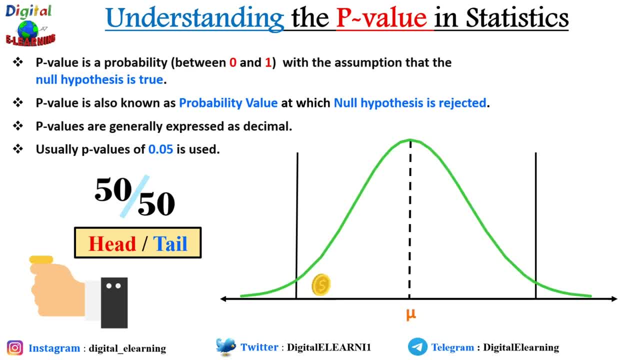 curve and on average we would expect to have 500 tails and 500 heads. but if i got 510 head and 490 tail, then do would you call this a fair coin or a unfair coin? but in this case we can say there is no sufficient evidence to suggest that the coin is fair or not. right? so if, again, if, if we get 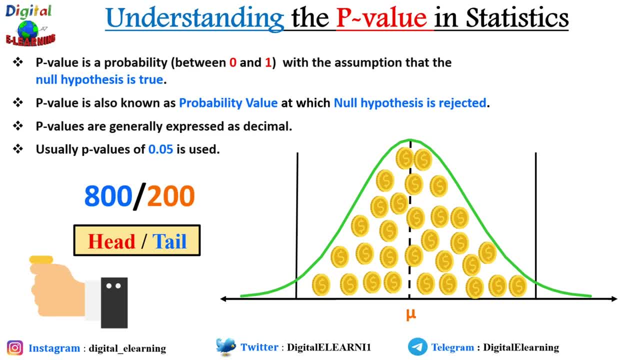 another case where we have 800 heads and 200 tail. would you still call this coin a fair coin? i guess we cannot call this a fair coin because we would have a strong suspect that this is an unfair coin and is biased towards the head. so in this case we would suspect the coin is biased. 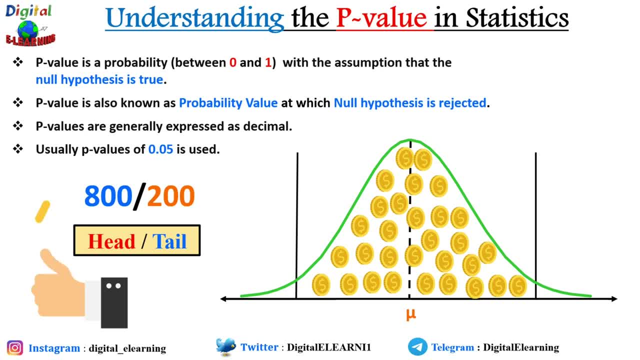 and this could be easily happen by chance. graphically, if you represent the p value, it is the area in the tail, that is the red area that i have marked. that is the distribution of your graphical distribution. my null hypothesis in this coin would be that my coin is fair and it should have equal probability. 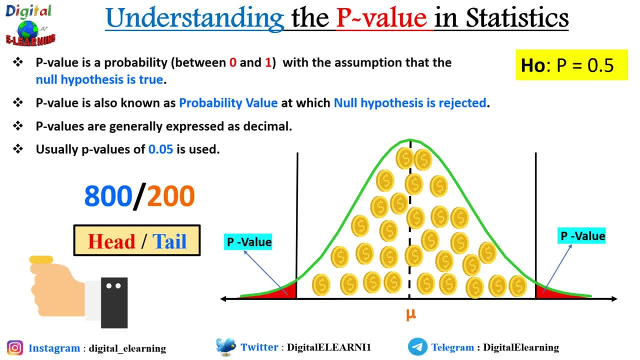 it is a default of worst case scenario. it is a known fact that it will have 50 percent head and 50 percent tail and my alternate would be: that is not 0.5. that is how you define the alternate and null hypothesis. in this case, the chance of occurrence of null and alternate are mutually. 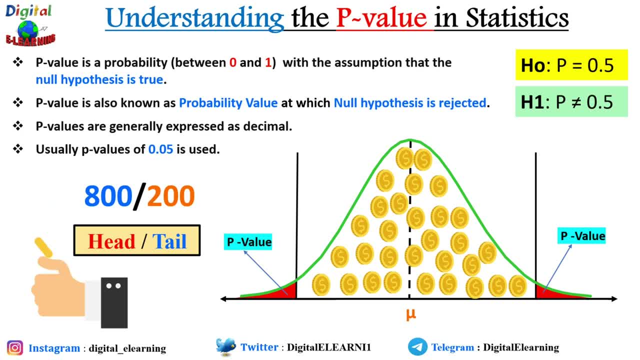 exclusive. this means then: either of them can occur. both cannot occur at same time. that is basic about the p value. now let us look at some decision rules. how do we- based on that, we will evaluate whether our result is significant or not- decision rules to understand the decision. 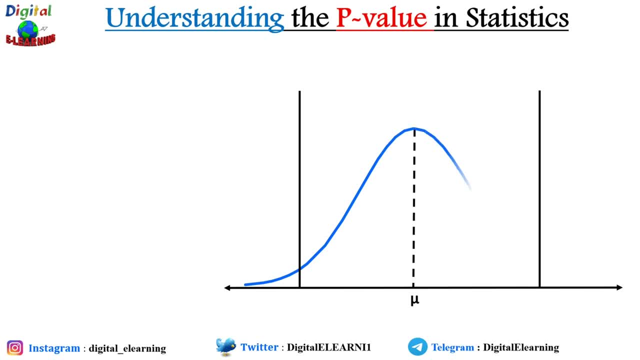 rules. let us first plot the normal distribution curve and these are my critical values. now, my first rule says: if p less than alpha- that is the significance level- then we can reject the null hypothesis. if it falls in this red region which is below the critical values, the term significance. 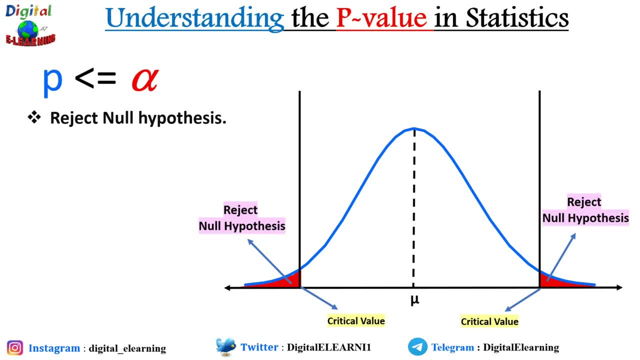 here means not anything major or important, but it just means the difference between two mean is not likely due to chance, and as the p gets further lower, the evidence allow you to reject the null hypothesis gets more stronger here. the second rule is if p is greater than alpha, that means we fail to reject the null hypothesis. 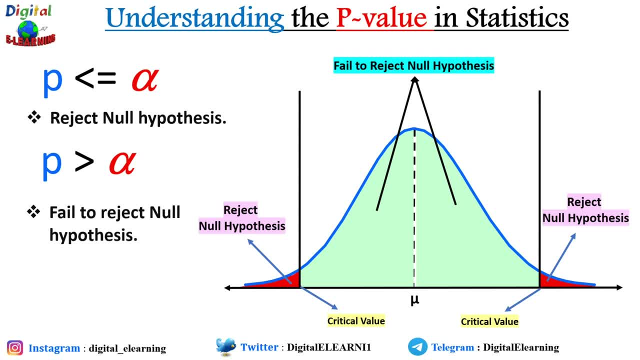 which falls in this green region. here the p value lies between 0 and 1. it won't reach exact 1 because in real life the group will probably not be exactly perfectly equal. and it also not reach 0 because there is always a possibility, even if it is extreme. so alpha here denotes the 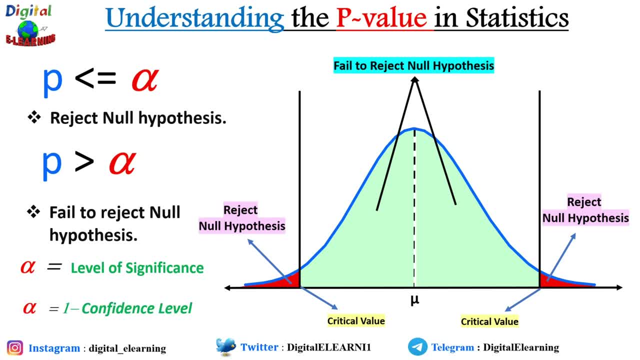 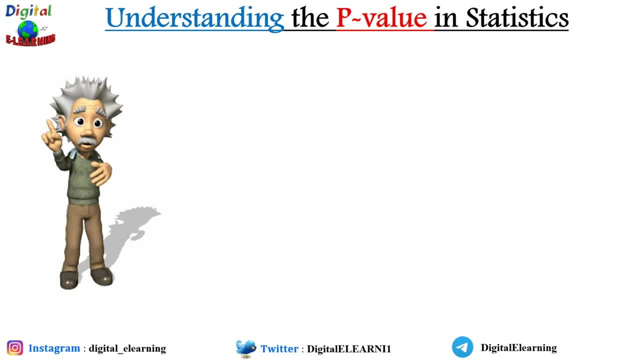 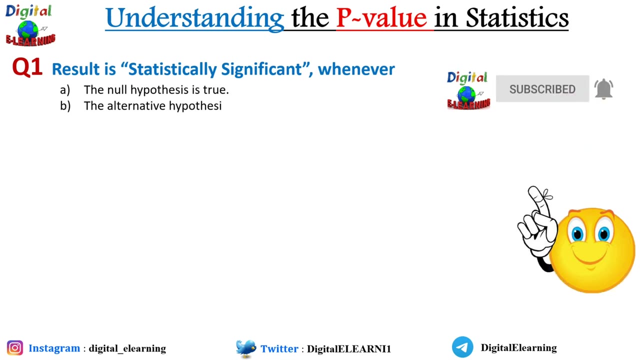 level of significance and how you calculate. you can create from 1 minus confidence level here. so before we start some numericals, let us do a quick check to understand how much you understood this concept till now. first question: the result is statistically significant whenever the null hypothesis is true, the alternate hypothesis is true, the p value is less than or equal to significant. 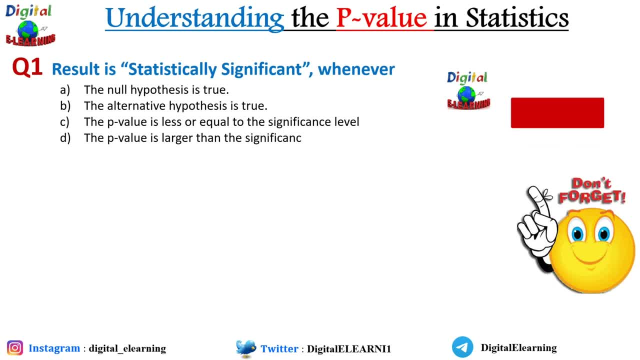 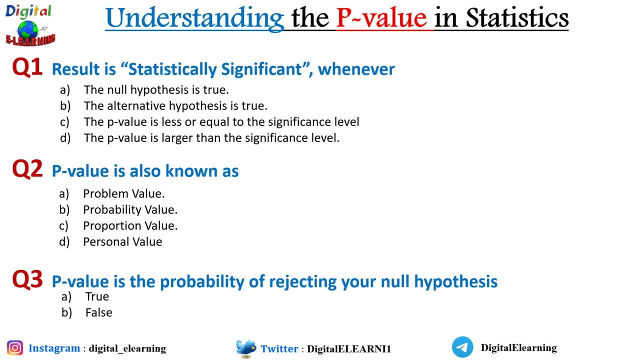 level, the p-value is larger than the significance level. second question: the p-value is also known as problem value, probability value, proportion value and the personal value. question three: p-value is the probability of rejecting your null hypothesis. is it a true statement or a false statement? you can leave your answers in the comment section below. 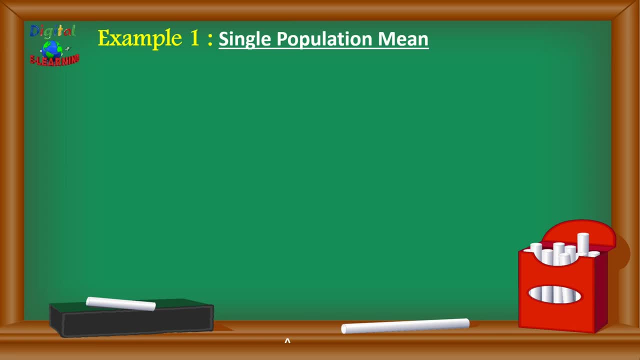 let's take the first example of single population mean. a vendor claims that the average weight of box is 1.84 kg. the customer randomly chooses 64 parts and find the sample weight as 1.88 kg. suppose the population standard division is 0.3 kg with alpha at 0.05. that is the level of. 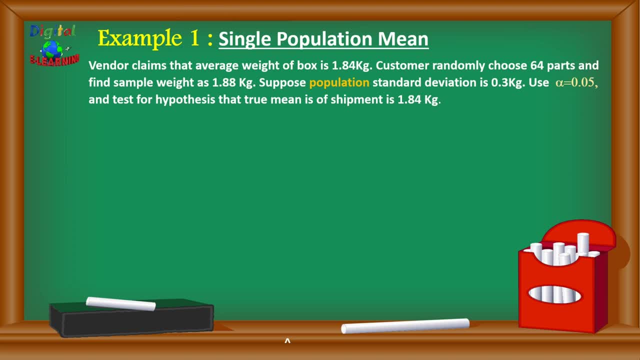 significance. we need to test for hypothesis that the true mean of shipment is 1.84 kg so we can find the sample weight as 1.84 kg. so our my null hypothesis is net mu is equal to 1.84 kg and our trend is it is not equal to 1.84 kg. 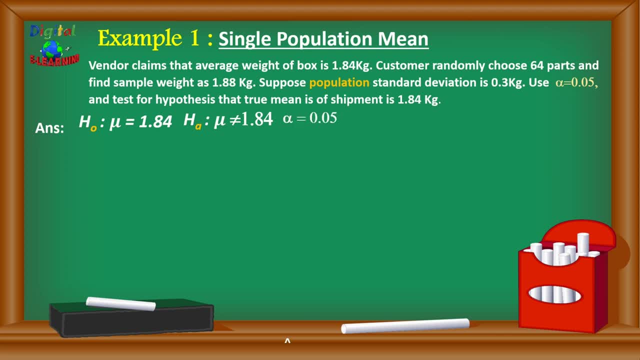 alpha, or level of significance, as 0.05. so let's plot it on that normal distribution curve. we mark it the area rejection area here. if it falls in the red region, we will reject the our null hypothesis. if it falls in between, we fail to reject the. 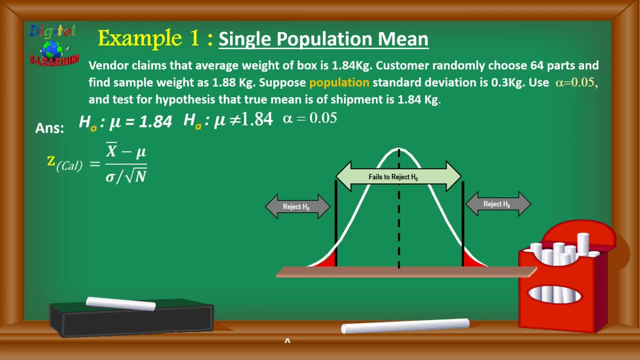 null hypothesis. so we can plot it on that normal distribution curve. we mark it the area rejection area here if it falls in between. we fail to reject the null hypothesis. so we'll use the Z formula, that null hypothesis. so we'll use the Z formula, that null hypothesis. so we'll use the Z formula. that is X power minus mu by Sigma by under root n. 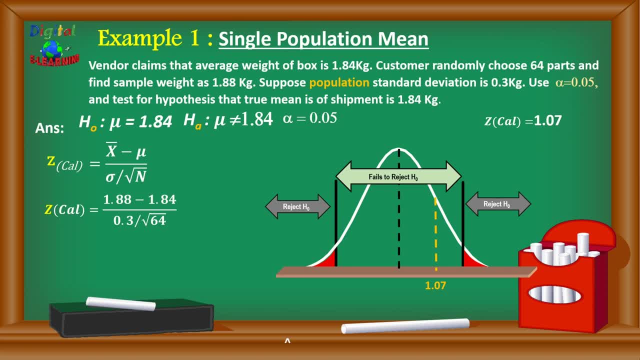 is X power minus mu by Sigma by under root n. is X power minus mu by Sigma by under root n. we'll put all this value here. we get Z. we'll put all this value here, we get Z. we'll put all this value here. we get Z calculated as 1.07. we go back to Z table. 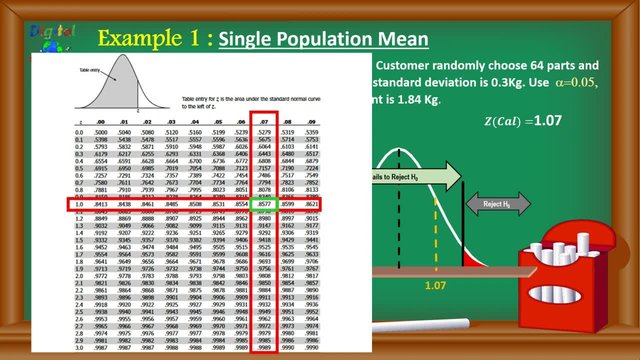 calculated as 1.07. we go back to Z table. calculated as 1.07. we go back to Z table. here we find out what is 1.07, so one. here we find out what is 1.07, so one. here we find out what is 1.07, so one from the Z table on the last column, and 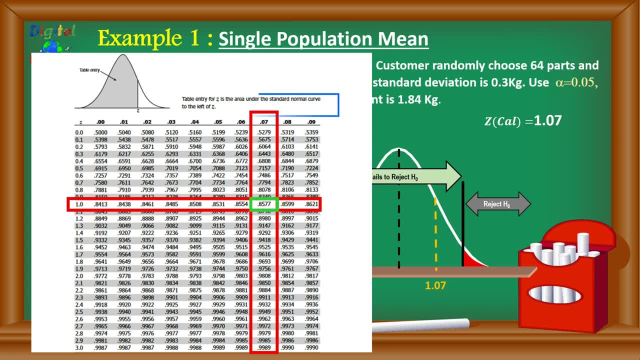 from the Z table on the last column and from the Z table on the last column and o7 from the vertical column, so we get o7 from the vertical column, so we get o7 from the vertical column, so we get 0.857. so this entry in this table is the. 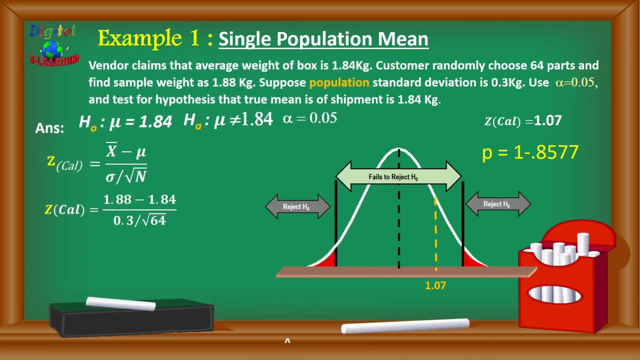 0.857. so this entry in this table is the 0.857. so this entry in this table is the standard normal curve to the left of the standard normal curve to the left of the standard normal curve to the left of the Z value. that means my. I'm getting P as. 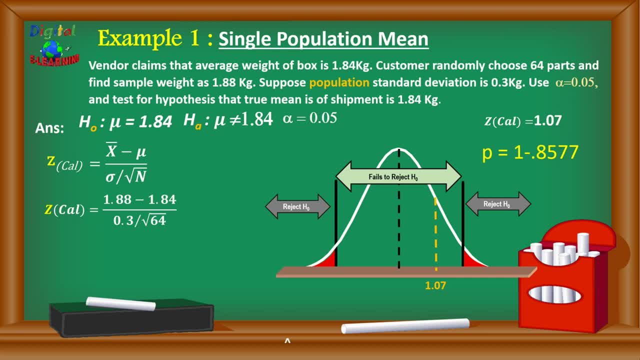 Z value. that means my I'm getting P as Z value. that means my I'm getting P as 1: 1 minus 0.8 577. this is the normal 1, 1 minus 0.8 577. this is the normal 1, 1 minus 0.8 577. this is the normal distribution is symmetrical, so area to 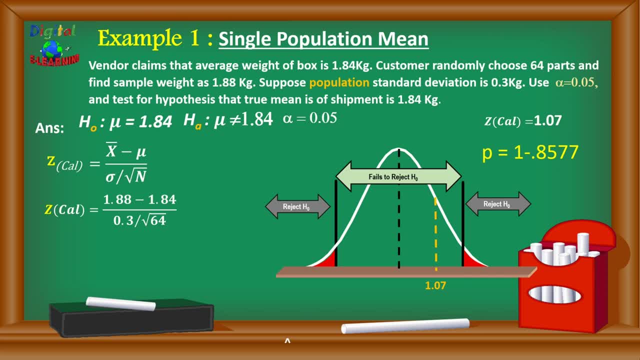 distribution is symmetrical, so area to distribution is symmetrical. so area to the right of the curve is equal to that. the right of the curve is equal to that. the right of the curve is equal to that of left. that is why we have to get it 1. 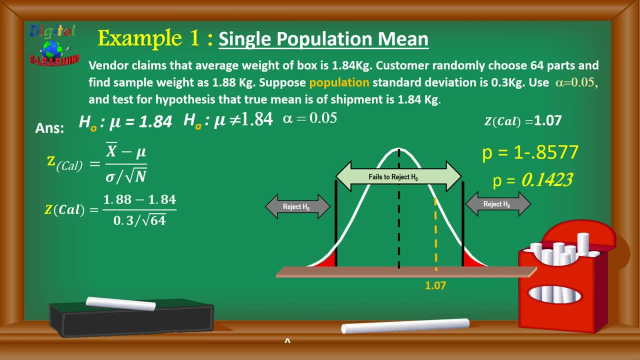 of left. that is why we have to get it 1 of left. that is why we have to get it 1 minus 0.85, and we get P as 0.1423, so in minus 0.85, and we get P as 0.1423, so in. 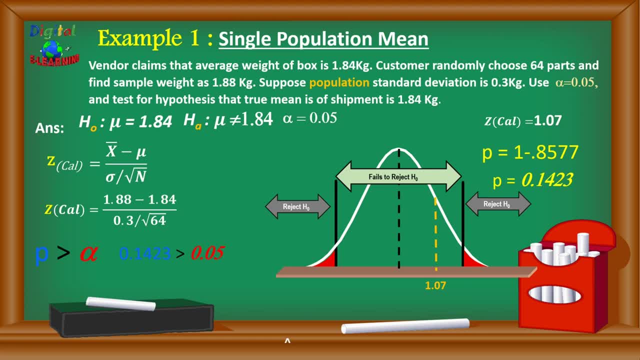 minus 0.85 and we get P as 0.1423. so in this case the my P is greater than alpha. this case the my P is greater than alpha. this case the my P is greater than alpha, that is, 1.4323 is greater than o5. so 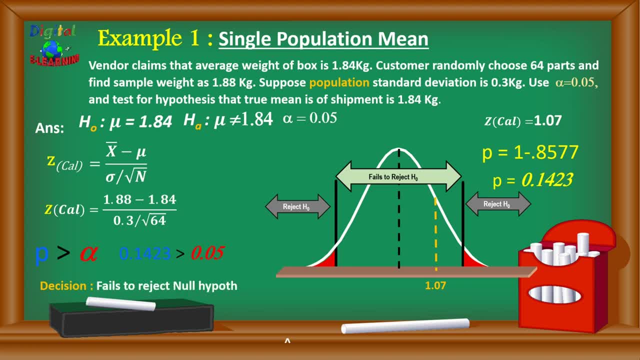 that is, 1.4323 is greater than o5. so that is, 1.4323 is greater than o5. so, since P is more than significance level, since P is more than significance level, since P is more than significance level, so we did this, then will be to fail to. 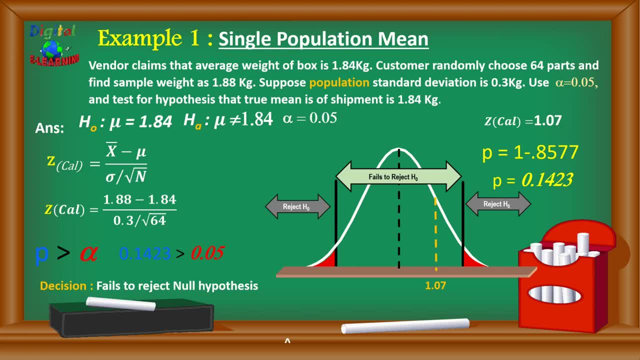 so we did this then will be to fail to so we did this then will be to fail to reject my null hypothesis here. this is reject my null hypothesis here. this is reject my null hypothesis here. this is how we do it, based on P value. let's take: 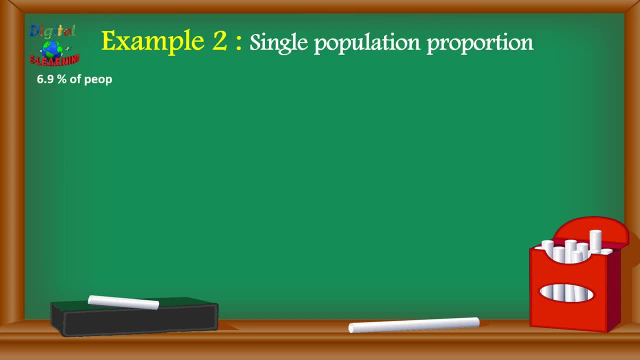 how we do it based on P value. let's take how we do it based on P value. let's take another example for single population. another example for single population. another example for single population proportion: six point nine percent of the proportion. six point nine percent of the. 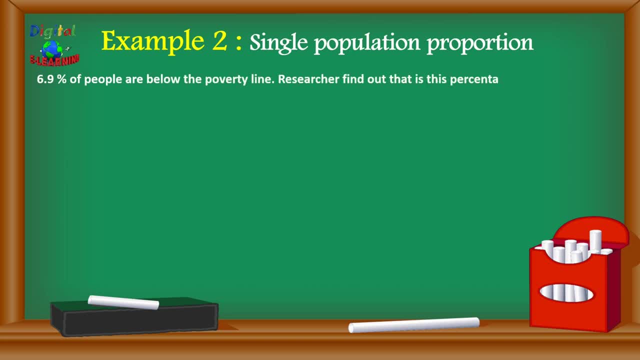 proportion. six point nine percent of the people are below the poverty line. people are below the poverty line. people are below the poverty line. researchers find out that this researchers find out that this researchers find out that this percentage is higher for their own percentage is higher for their own. 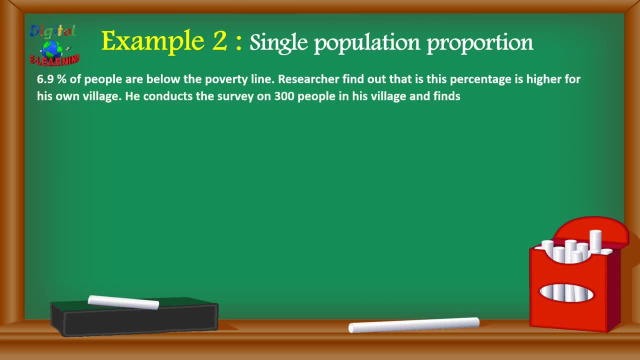 percentage is higher for their own village. he conducts a survey on 300 village. he conducts a survey on 300 village. he conducts a survey on 300 people in his village and find out that people in his village. and find out that people in his village and find out that 30 out of 300 are below the poverty line. 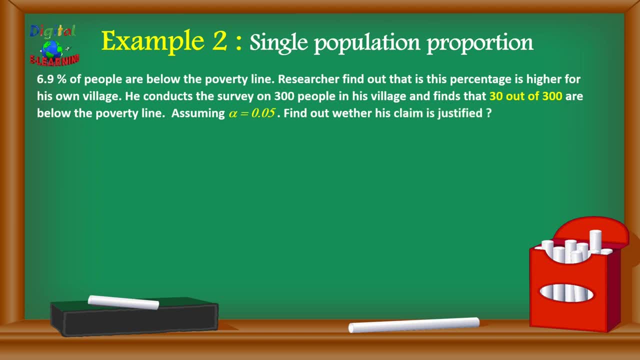 30 out of 300 are below the poverty line. 30 out of 300 are below the poverty line, assuming the alpha of 0.05. we have to. assuming the alpha of 0.05. we have to. assuming the alpha of 0.05. we have to find out whether his claim is justified. 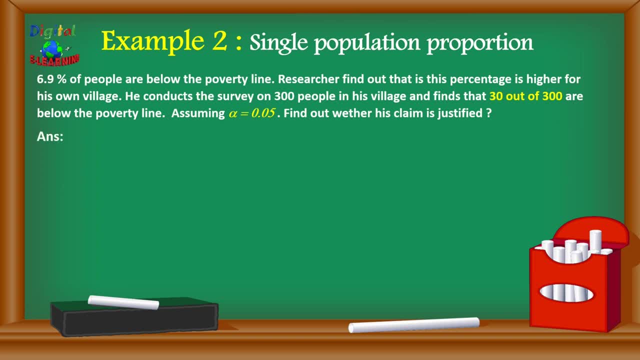 find out whether his claim is justified. find out whether his claim is justified or not. so my null hypothesis is P naught or not. so my null hypothesis is P naught or not. so my null hypothesis is P naught equal to 0.069, which is coming from 6.9. 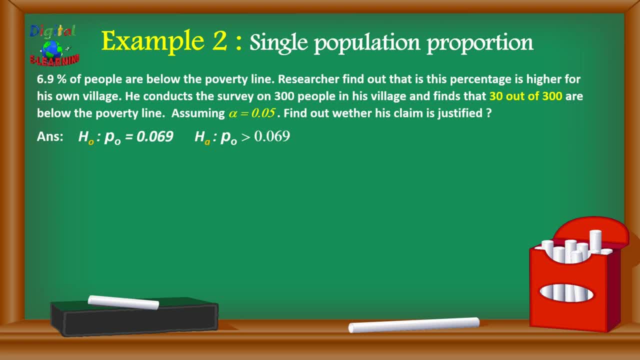 equal to 0.069, which is coming from 6.9. equal to 0.069, which is coming from 6.9 percent of the population. alternate percent of the population. alternate percent of the population. alternate hypothesis is: P naught is greater than. 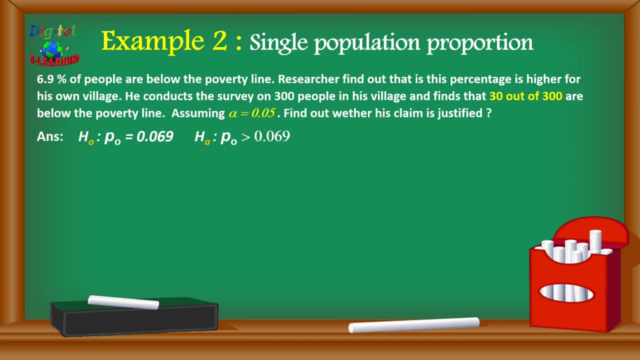 hypothesis is P naught is greater than. hypothesis is P naught is greater than 0.069, since the claim is that his 0.069. since the claim is that his 0.069, since the claim is that his percentage is higher in his village. so 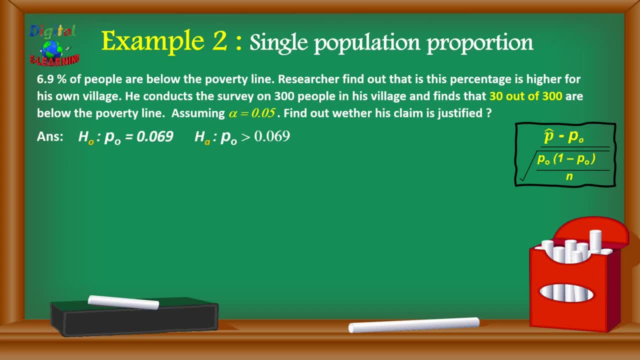 percentage is higher in his village. so percentage is higher in his village. so we use this formula for calculating Z. we use this formula for calculating Z. we use this formula for calculating Z: calculated, that is P hat minus P naught. calculated, that is P hat minus P naught. 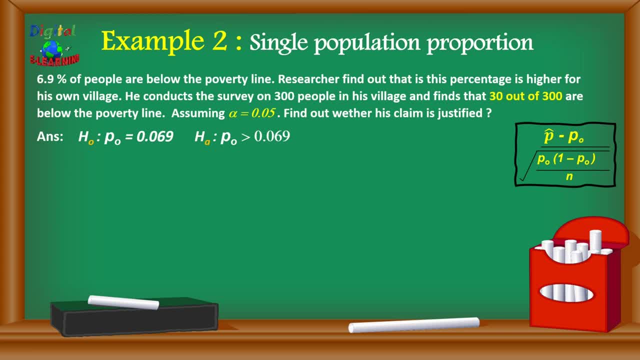 calculated, that is: P hat minus P naught, divided by under root of P naught into 1. divided by under root of P naught into 1. divided by under root of P naught into 1, minus P naught, divided by n, where P naught. 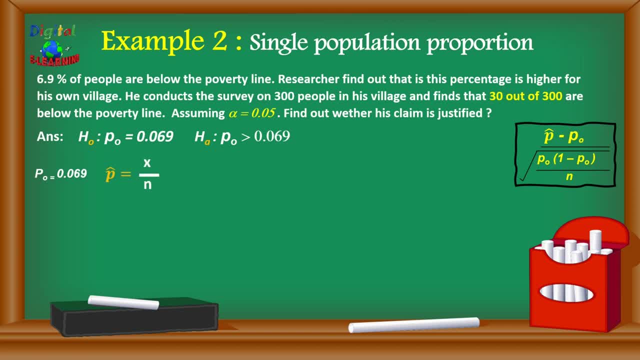 minus P naught divided by n, where P naught minus P naught divided by n, where P naught is equal to 0.069 P. hat is X squared by is equal to 0.069 P. hat is X squared by is equal to 0.069 P. hat is X squared by n, so X is 30, the result that he got out. 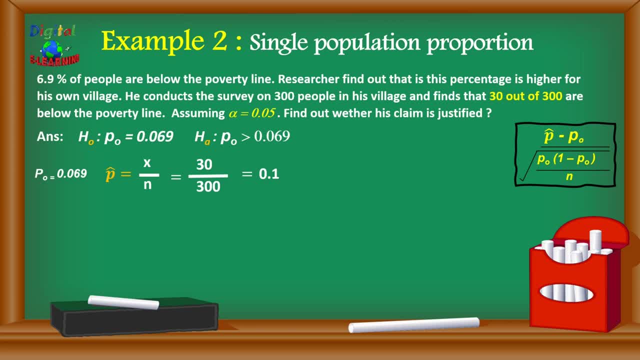 n, so X is 30. the result that he got out n, so X is 30. the result that he got out of 300 samples in his village and P hat of 300 samples in his village and P hat of 300 samples in his village and P hat is coming as 0.1. now we'll put these: 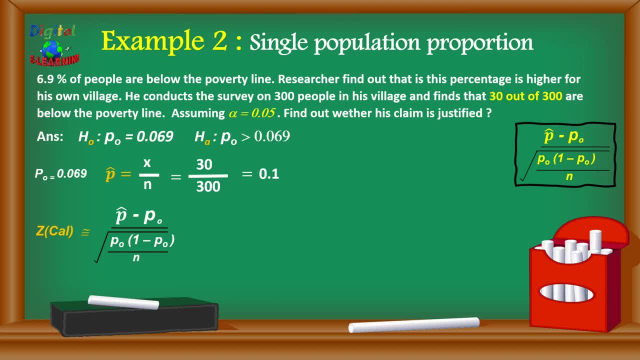 is coming as 0.1, now we'll put these. is coming as 0.1. now we'll put these values in of P. hat P naught in the Z values. in of P. hat P naught in the Z values. in of P. hat P naught in the Z colored formula. we get Z calculated as 2. 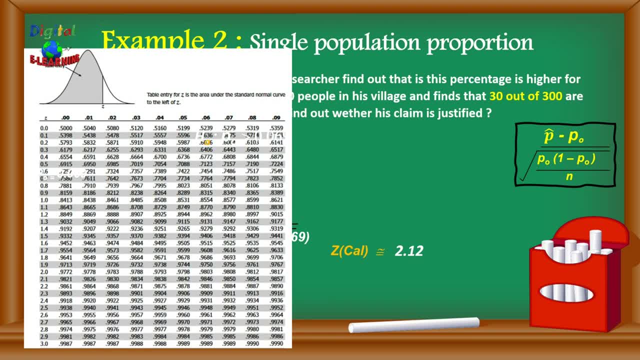 colored formula: we get Z calculated as 2. colored formula: we get Z calculated as 2. point 1, 2 and go back to C table. but point 1, 2 and go back to C table. but point 1, 2 and go back to C table. but first let us plot this in the normal. 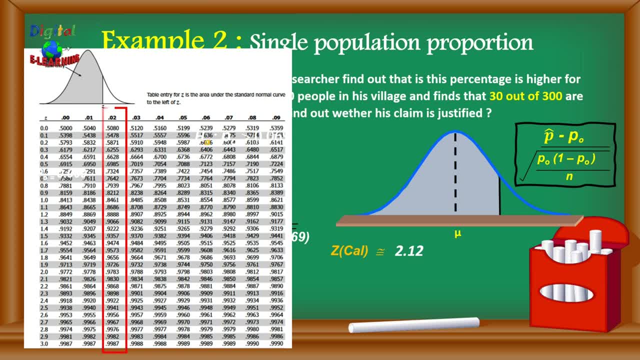 first, let us plot this in the normal. first let us plot this in the normal: distribution curve: distribution curve: distribution curve. in the Z table, we'll find out 2.12. in the Z table, we'll find out 2.12. in the Z table, we'll find out 2.12, which comes at the intersection of 2.1. 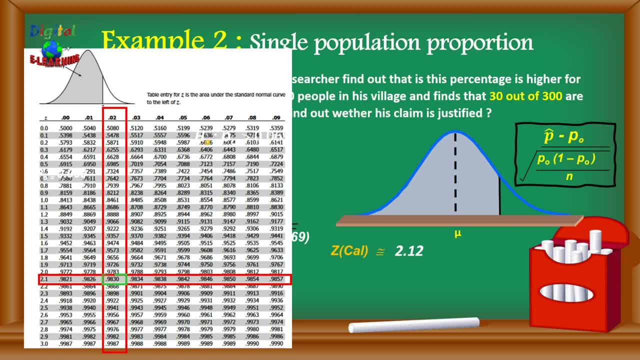 which comes at the intersection of 2.1, which comes at the intersection of 2.1 and 0.02 and 0.02 and 0.02. we get 0.9830, so this 0.9830, so this 0.9830. 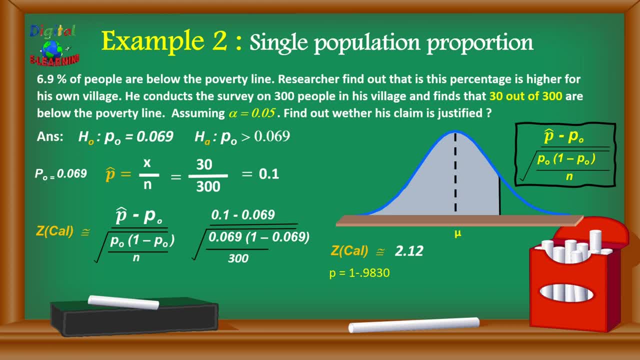 so this 0.9830- uh, this area under the curve is one. we uh, this area under the curve is one. we uh, this area under the curve is one. we subtract it from one, subtract it from one, subtract it from one. so we get p as 0.017. 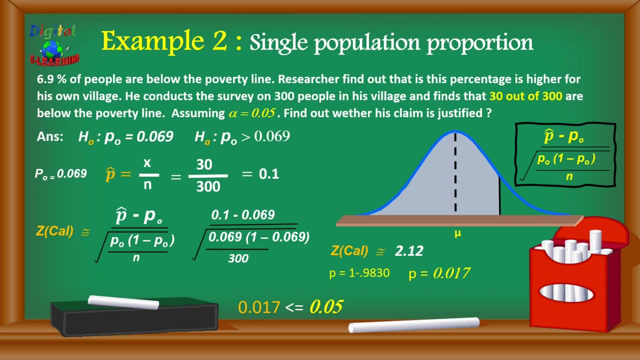 so we get p as 0.017, since this this 0.07 is less than 0.05. since this this 0.07 is less than 0.05, since this this 0.07 is less than 0.05 than the significance level alpha. 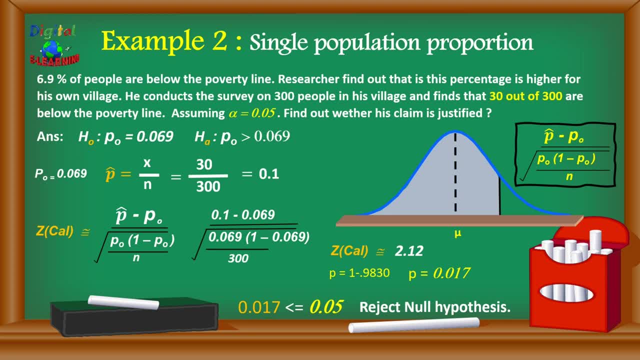 than the significance level alpha than the significance level alpha. so we reject the null hypothesis in. so we reject the null hypothesis in. so we reject the null hypothesis in this case, this case, this case. this is another example of p value. this is another example of p value.